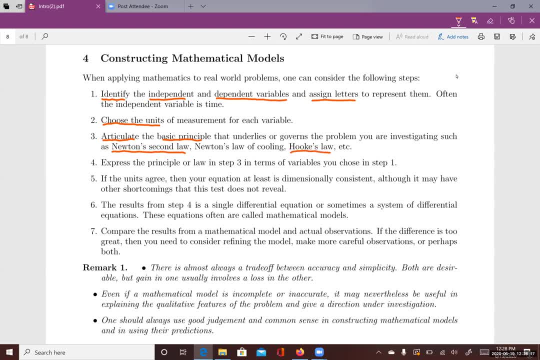 And you can use Hooke's laws if you're trying to measure the precisions of springs and so on and so forth. So use some principles that you have known And that you can use with the directions of your investigations. One of the next steps is once you identify your variables, once you identify the principles. 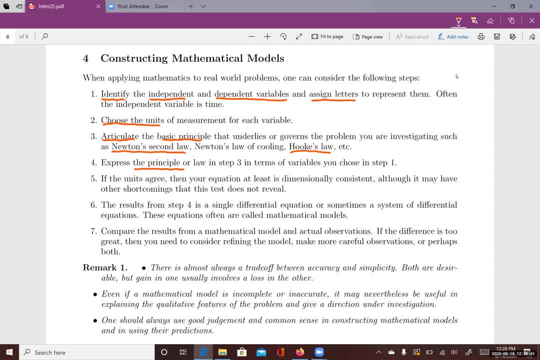 then you express those principles or the law in step number three here in terms of the variables that you chose in step one. So just going to line up your principle, the principle, the laws that you're using, with the variables that you identified for your problem. 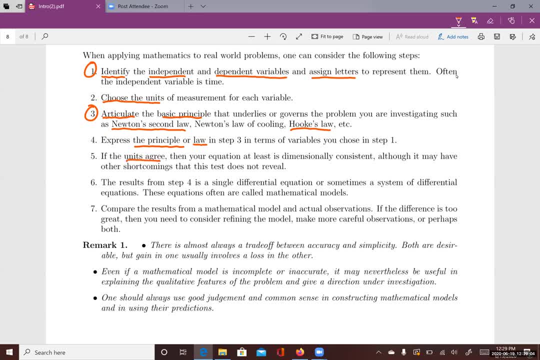 If the units agree, then your equations right, at least dimensionally consistent. Or if the units do not agree, then you have to go back to your, either your variables or the principles in order to like, match them up. Make sure that all the units agree. 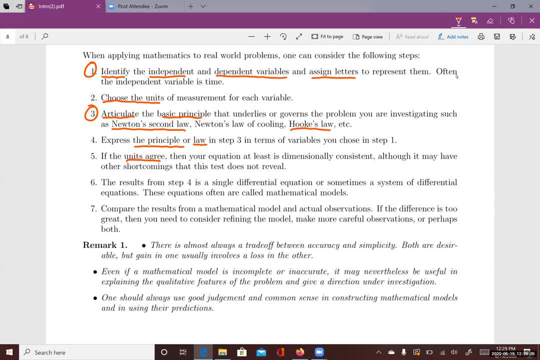 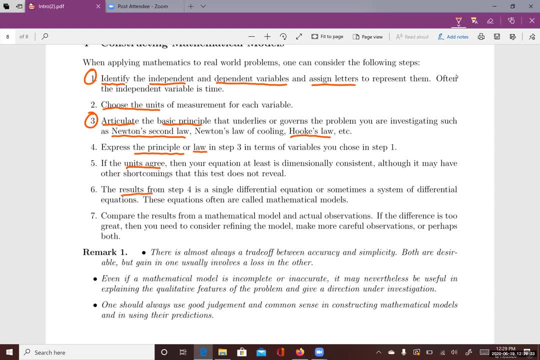 And then you have to go back to your either your variables or the principles in order to, like, match them up. Okay, Okay. Well then the result that you get from step number four here will give you either a single differential equations, if you only have one outcome, like one unknown functions, or sometimes, 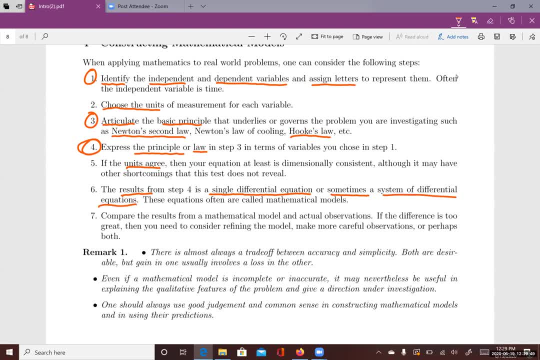 you will get a system of differential equations. if you have multiple unknown functions, Okay, Okay, Wonderful, Thank you very much. is too big, too great, then you need to either consider to refine your model, adjust parameters right of the models or make more careful observations or make more observations. 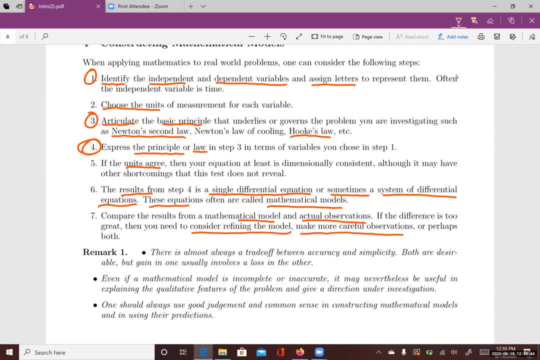 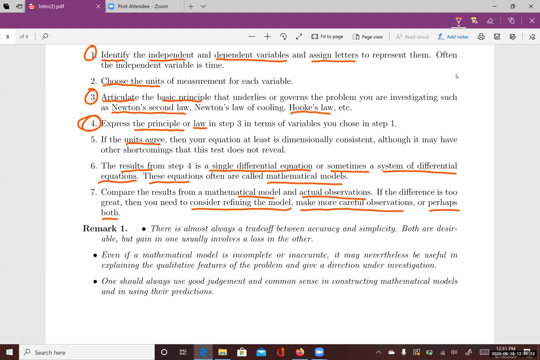 or more careful observation, or sometimes, perhaps, do both, Go back, adjust your model, make more careful observations. So then, the difference between mathematics models, mathematical models and actual observation is not so big. Well, there's some remarks that you want to keep in mind when you use mathematics to model some natural phenomenons. Well, there's. 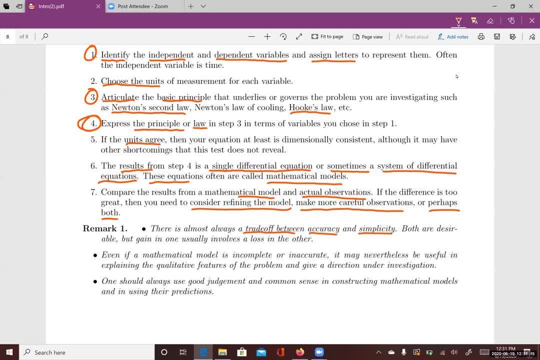 always a trade-off between accuracy and simplicity. You want to build your model so it can be accurate, fit your actual observations, but at the same time you want to keep your model simple, because the simpler your model is, the better, the easier you. 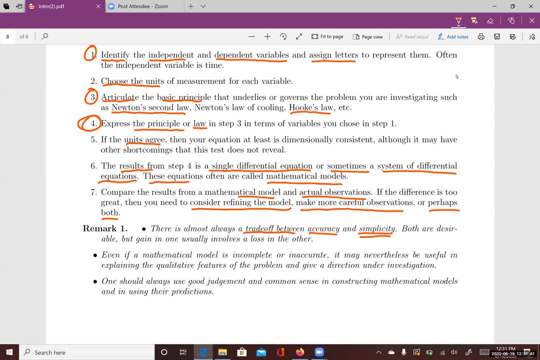 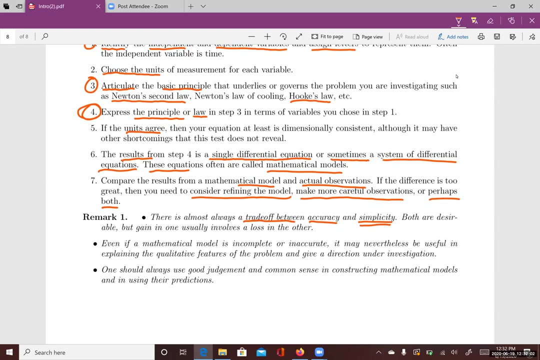 can adjust your model if you are running into errors, difference between models and actual observations, So keeping both. both, like, accuracy and simplicity are desirable. You have to like make a trade-off between the two, but the gain in one usually involves the loss of the other. okay, Well, sometimes even if the 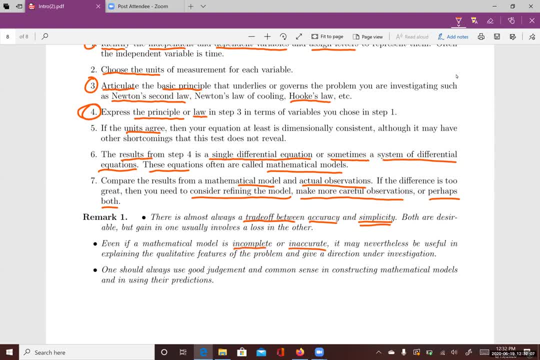 mathematical models is incomplete or inaccurate, right when you compare it with actual observations, but it still, you know. give you some directions or we use some explanations of the qualitative features of the problems that you are tackling. So give some directions, some qualitative features under your investigations. 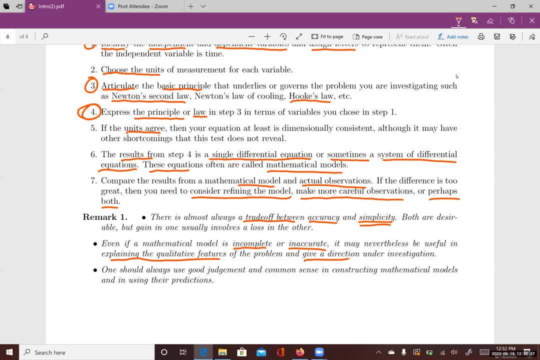 Okay, and lastly, you should always use good judgment and common sense when you're constructing mathematical models and when you use their predictions. So you try your best to come up with some models that align with actual observations. right, But again, the observation that you're collecting, 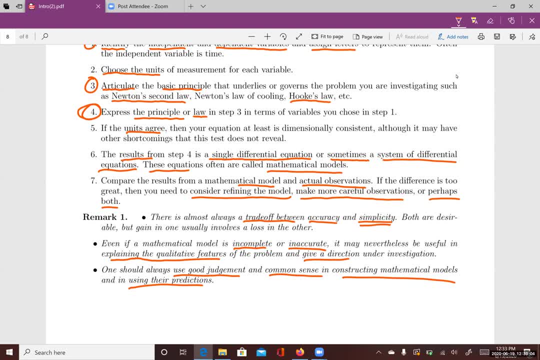 is the it can be called historical observations. You have to make sure that you should make sure think about whether your models will be good, will be applicable when you apply those model in future observation. So it's always have good judgments, the balance between the two.